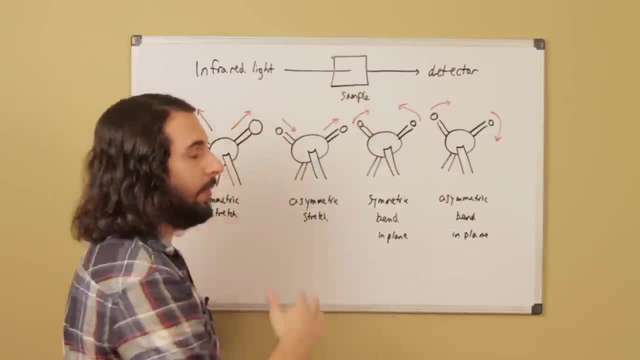 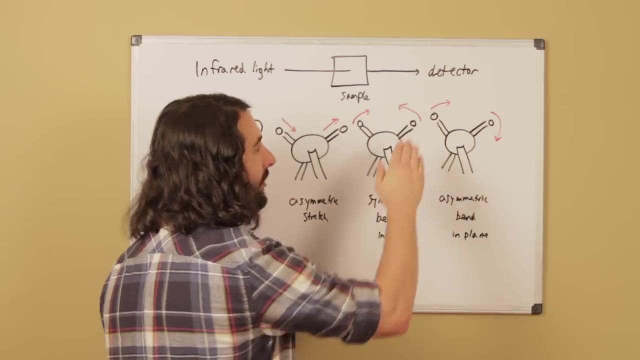 We irradiate a molecule. We're going to take a sample with infrared light. That light is going to interact in some way with the compounds in the sample And then it will eventually reach a detector. So some light will be absorbed by the sample, some will not, some will pass through. 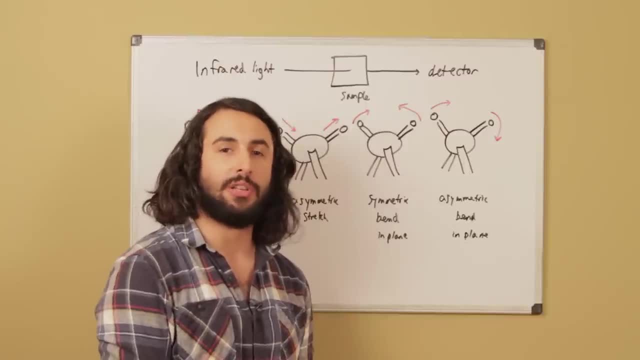 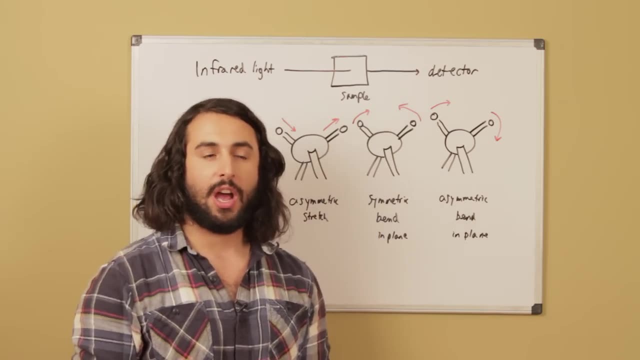 And this is information that we can use to figure out something about the structure of the molecule. The reason that we use infrared light is because different molecules. we already know that molecules move around. They have translational motion. We know that heat energy is converted into carbon. 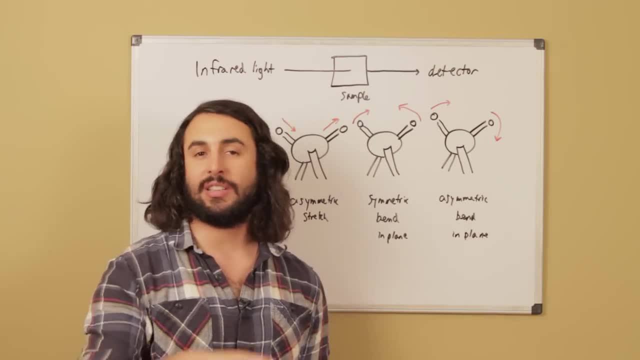 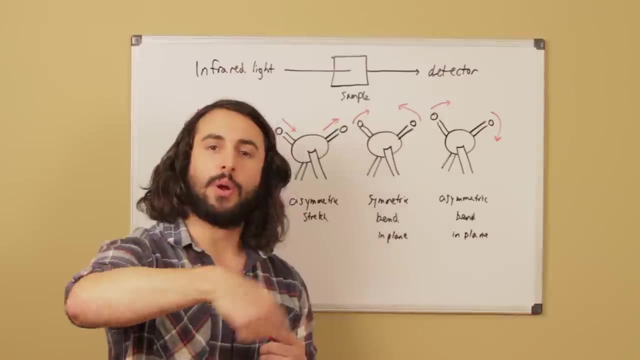 We know that kinetic energy of motion- So molecules, let's say in a gas or even in a liquid, are moving around with respect to one another. And through conformational analysis we also know that bonds are rotating all the time. So there is rotational motion for all of the sigma bonds. 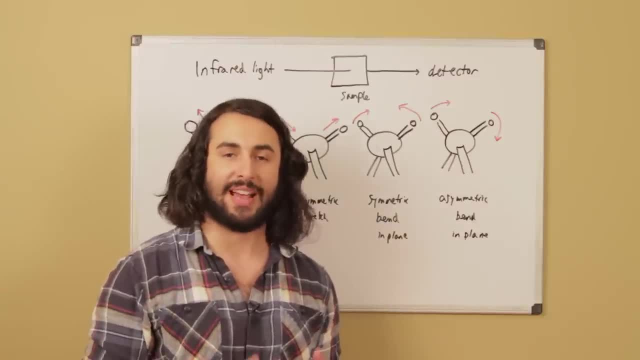 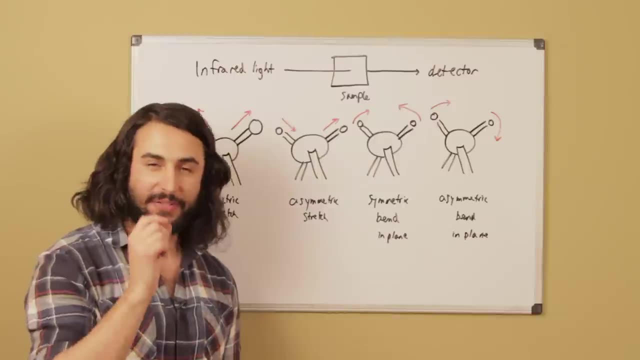 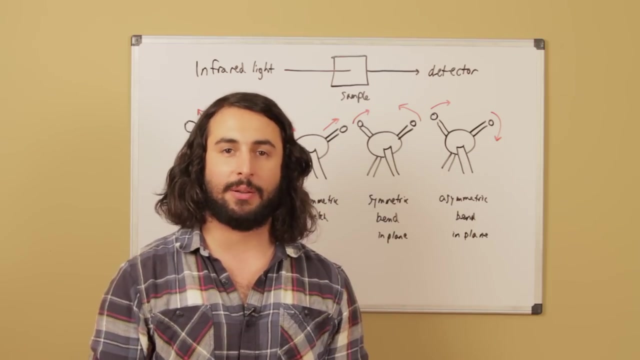 But chemical bonds are also doing other things. as it happens, They can do these other things that occur specifically when they are irradiated with a very specific wavelength of infrared light. They can do something like a symmetric or an asymmetric stretch. So let's say, my body is the central atom and these are two atoms that it is bound to. 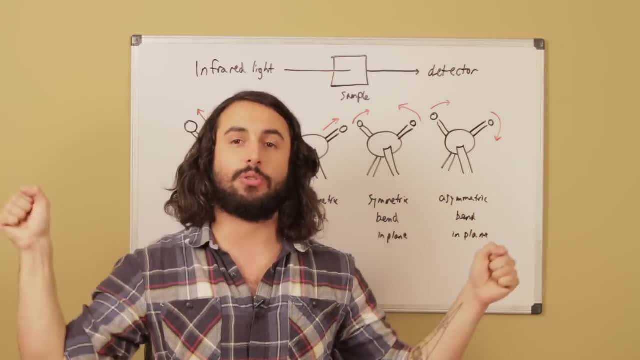 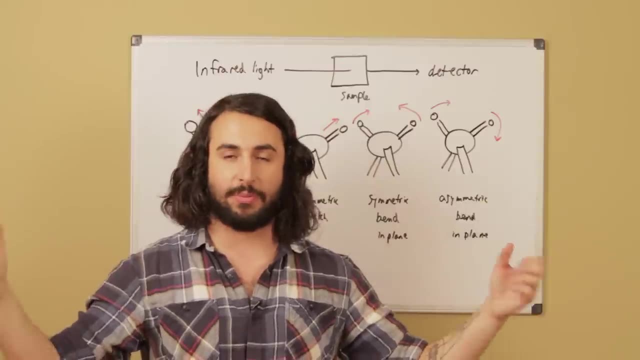 And so my arms are covalent bonds, And so this would be a symmetric stretch. The covalent bonds can actually be contracting and expanding at a particular vibration, depending on whether it has absorbed this particular photon of UV light. So this is a symmetric stretch. 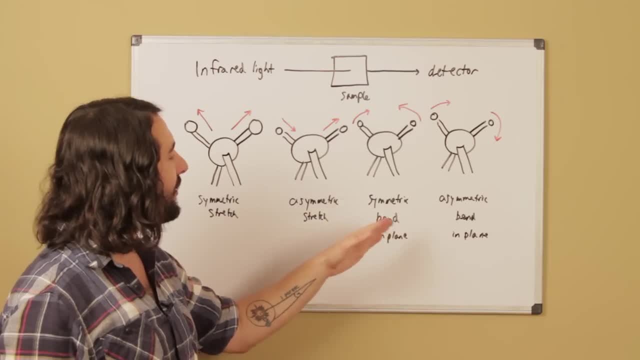 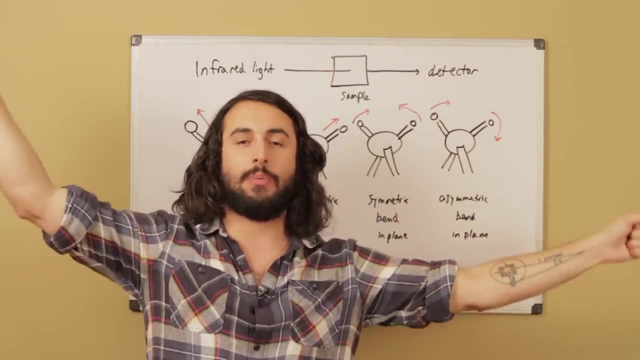 This would be an asymmetric stretch, And we can also have a symmetric bend or an asymmetric bend in plane. So that would look like this: This would be symmetric or we could have asymmetric, And we can actually have twisting. We can have it like this, which would be symmetric or it would be. 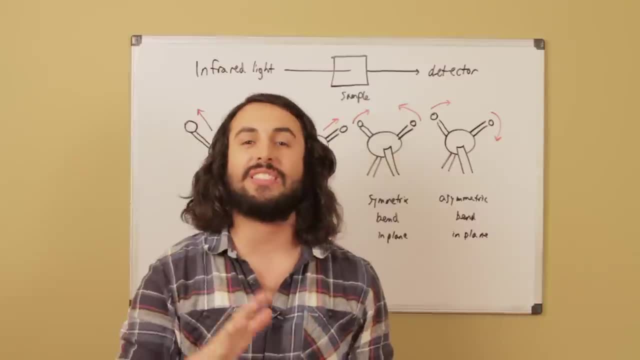 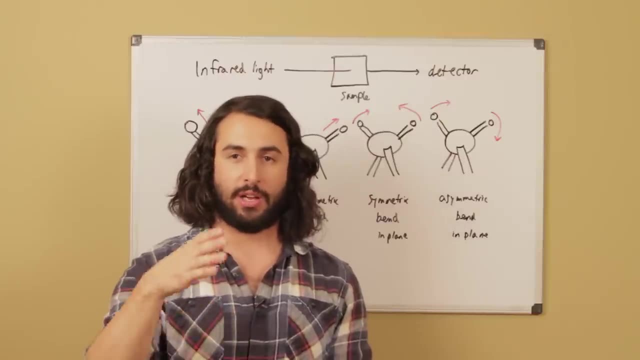 I can't even do it. It's very difficult to do. But the point is we have all of these different kinds of vibrational motions happening in a molecule And they occur at very particular energies. So they will occur when a wavelength of a very specific infrared light is absorbed. 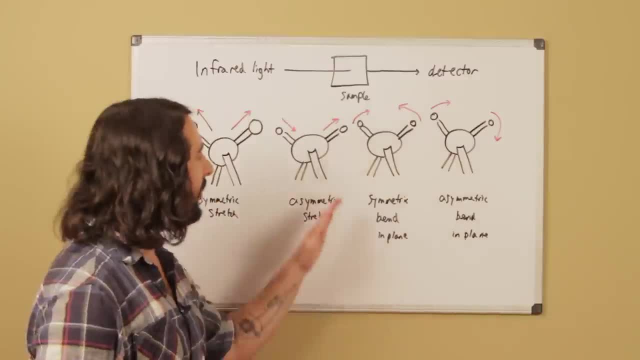 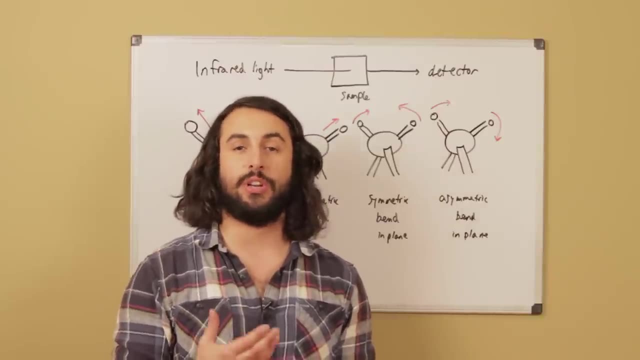 And it will vary depending on the functional group. So the identity of these atoms will affect the photon of absorption. So this is information that we're going to use to generate an IR spectrum. So let's look at what that looks like right now. 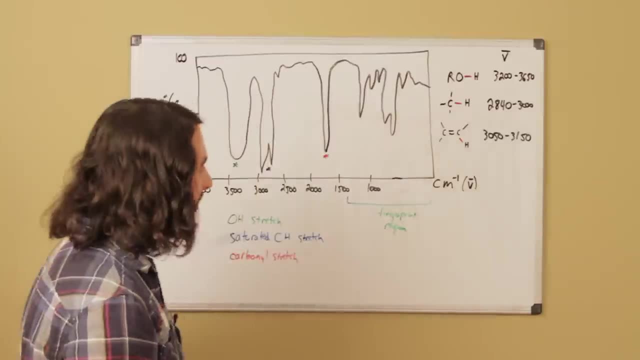 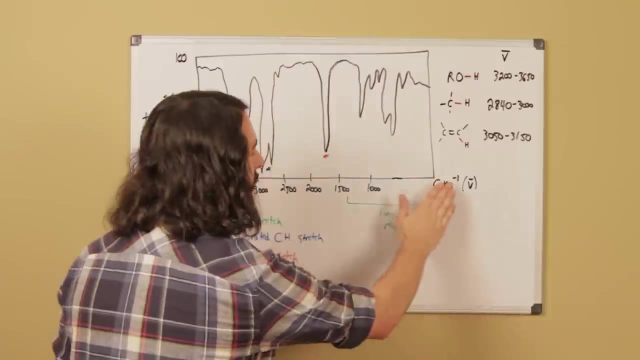 Okay. so what I've done here is I've drawn a sample IR spectrum, So let's take a look at what these look like and try to understand what we can use them for. So let's look at the axes. First, on the bottom here we have the wave number. 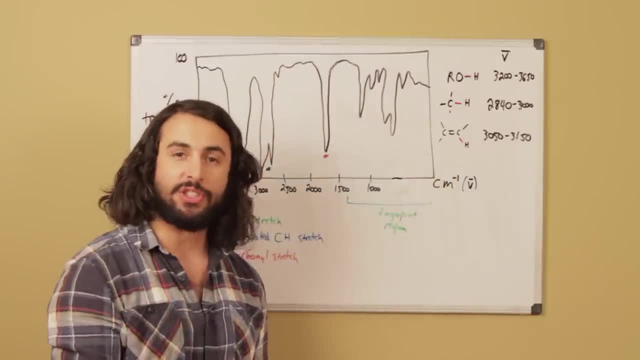 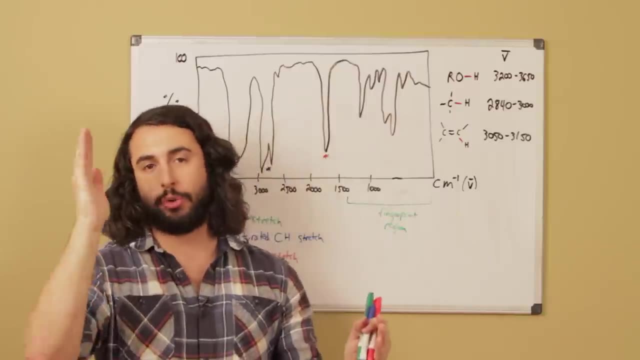 The wave number is telling us about the very particular wave number, The particular energy of infrared light. So infrared light is a certain band, It's a certain part of the electromagnetic spectrum All the way from this wavelength to this wavelength. So there are many energies of infrared light in between. 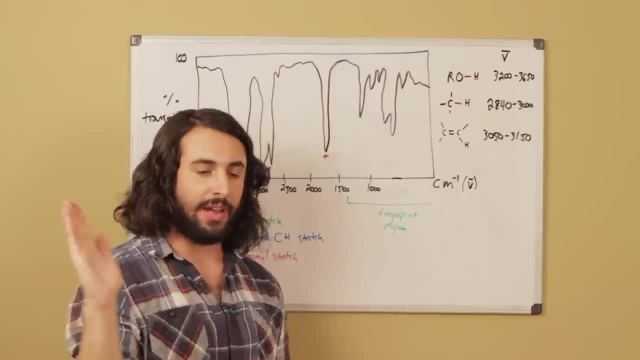 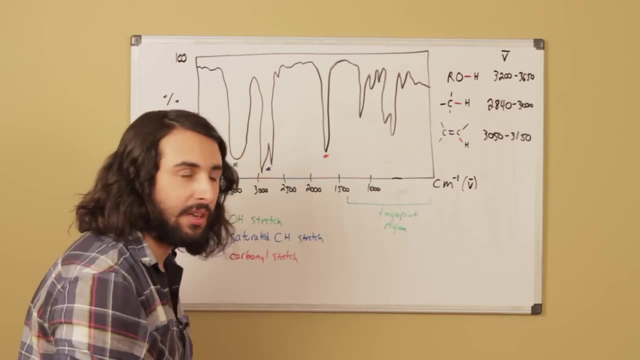 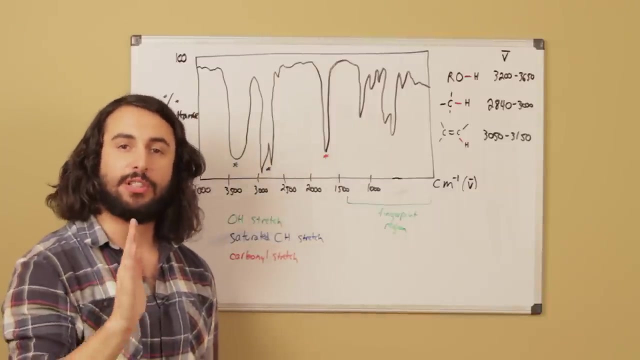 And so we're irradiating our sample with all of this infrared light, of all of those different wavelengths, And so the wave numbers here are the way we differentiate between those individual energies of IR radiation. On this axis we have the transmittance or the percentage of that particular wavelength. 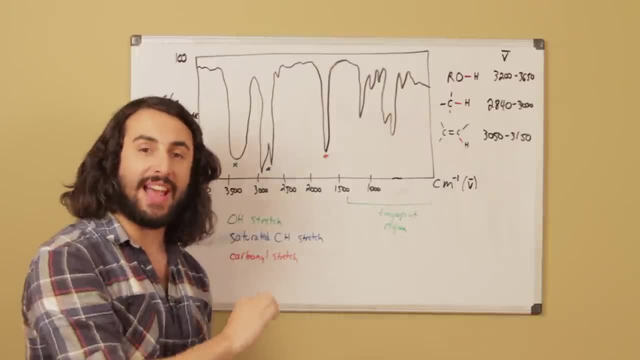 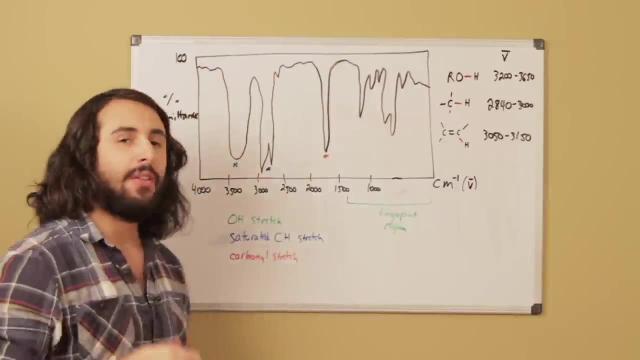 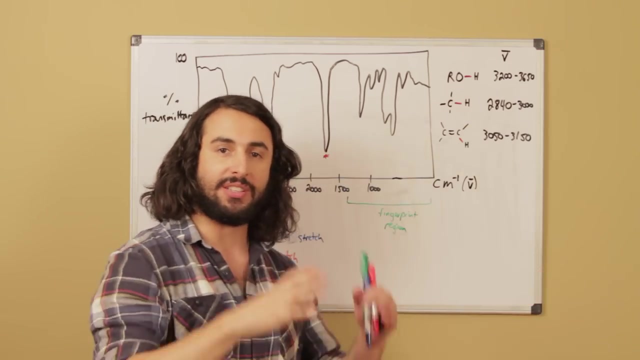 Or that particular wave number rather, That reaches the detector. So if we have information at 100% or near 100% transmittance, That means that IR light that corresponds to that wave number is all getting through. It's all getting through the sample. 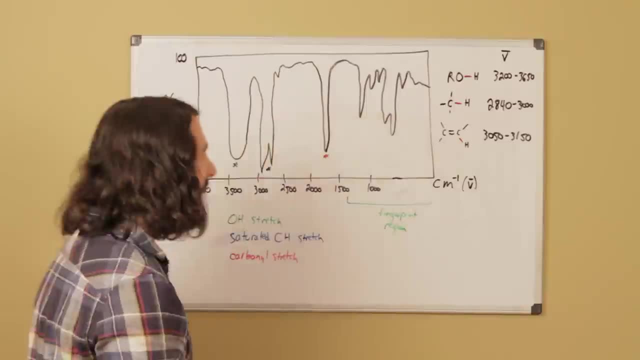 It is not being absorbed by the sample, It's going to make it to the detector And then where we have peaks here where we have information. So let's look at this wave number right here. Whatever is going on with IR light of this particular wavelength? 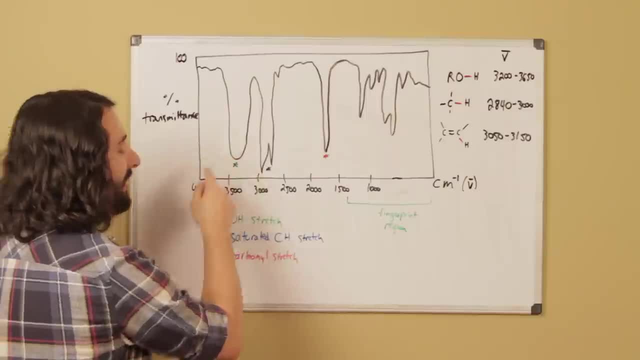 Whatever is going on with IR light of this particular wavelength? Whatever is going on with IR light of this particular wavelength, It is not making it to the detector. We can see that it has a very low percent transmittance. And if it is not making it to the detector, 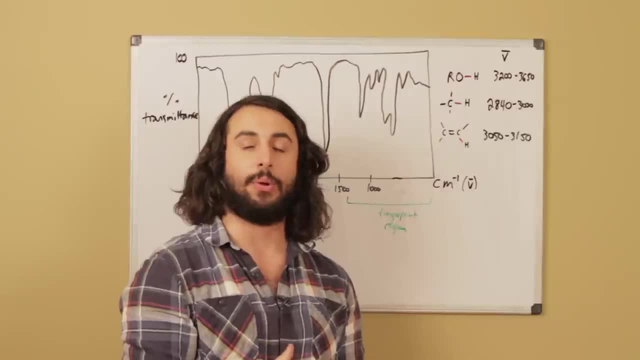 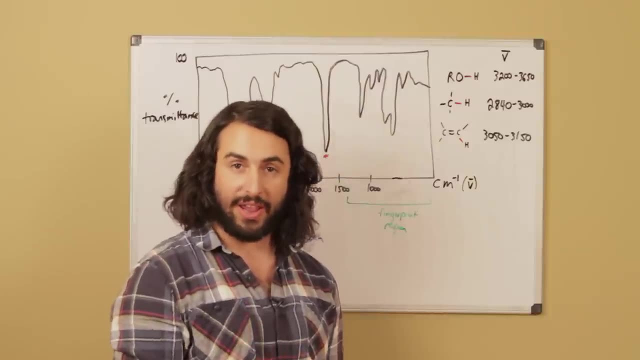 It is being absorbed by something in the sample. So there is a particular functional group in the molecule that is in the sample That absorbs IR light of that wavelength And that is information that tells us about what kind of bonds are in that compound. 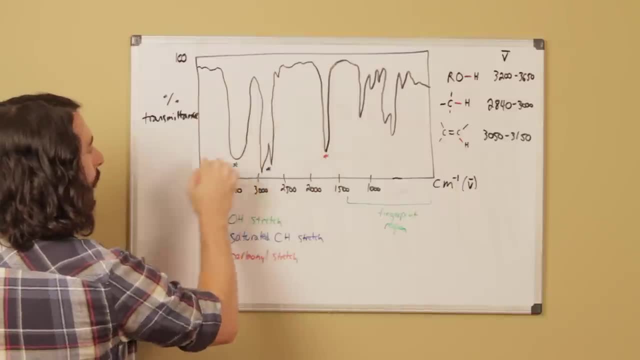 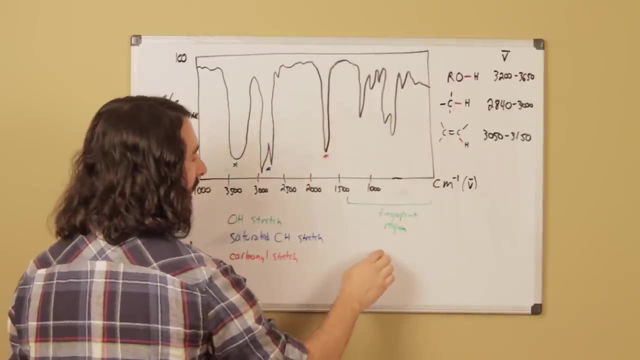 So looking across here, we can see that here's some important data. Here's some important data, important data. we should note that this region here around 1500 and below, is called the fingerprint region. there's some very delicate information there, but 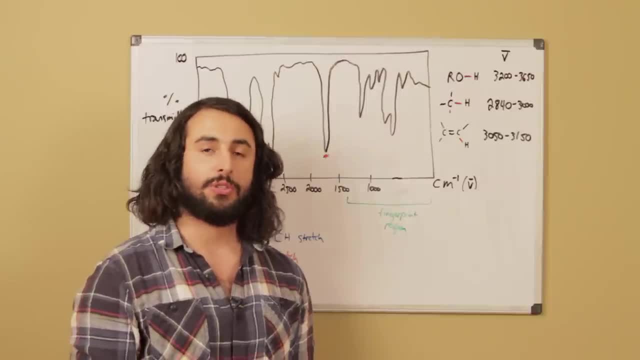 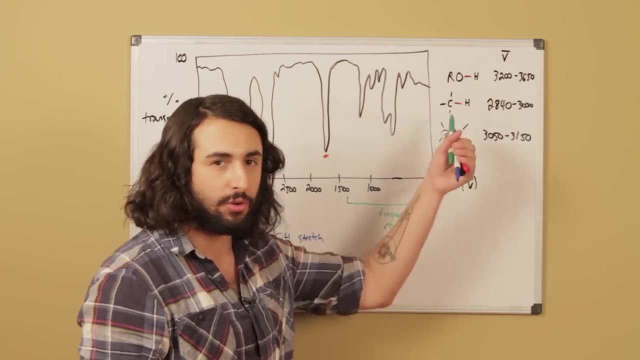 it's very complicated to analyze and it goes beyond the scope of this tutorial, so we won't talk about the fingerprint region right now. but what we want to understand is that we have tables. now I've only written three things up here, but there's long tables of every functional group that we 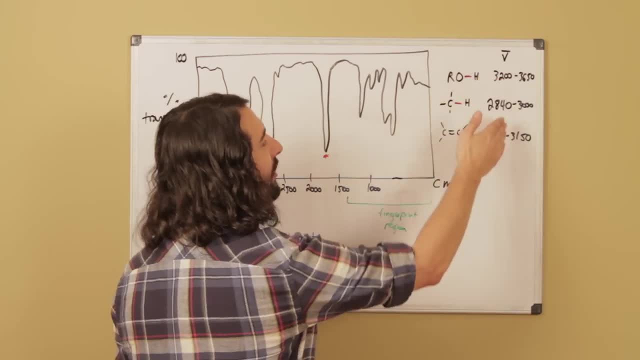 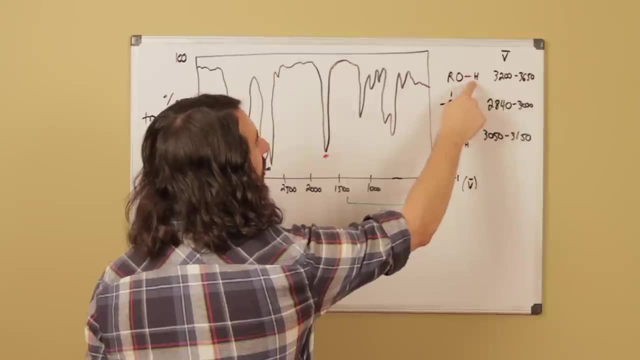 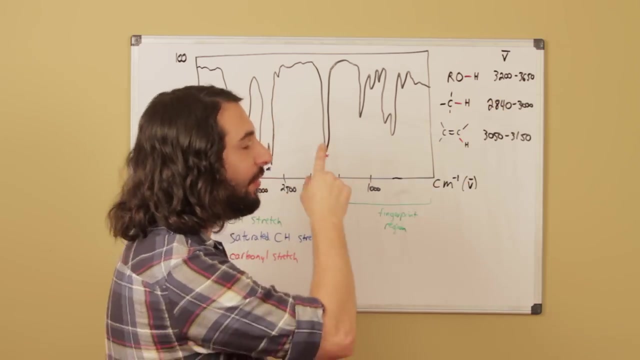 can imagine in a molecule and we can talk about the particular wave number of IR light that is absorbed by that functional group. so for example, we have the OH-Sigma bond. right here the OH stretch occurs at this wave number. so if that oxygen-hydrogen covalent bond absorbs infrared light of that, 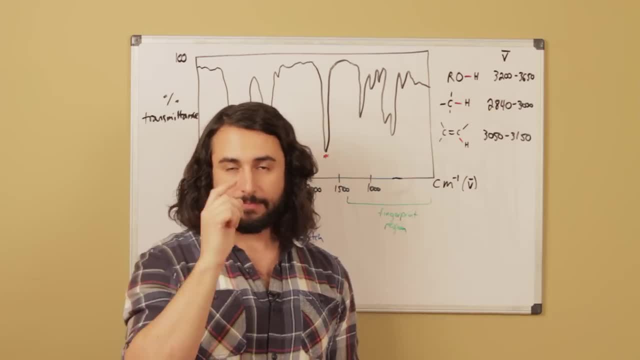 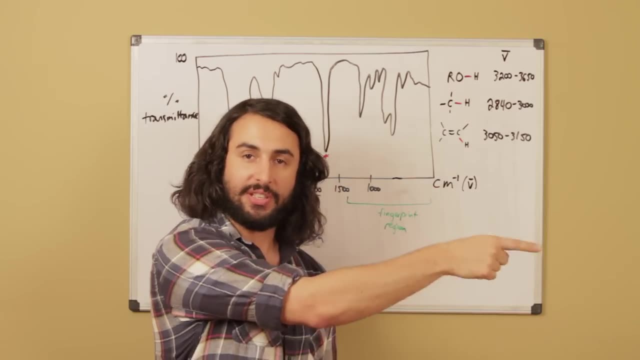 particular wave number, it will begin to stretch like this and if it does, if it is irradiated with light of that wave number, it is being absorbed, which means it does not get to the detector, and that's why we see something like this. so we call this the OH stretch, and 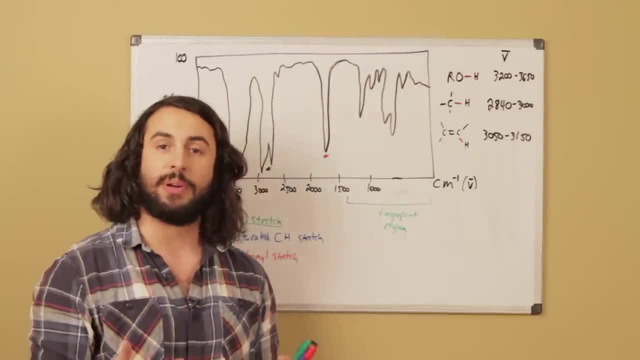 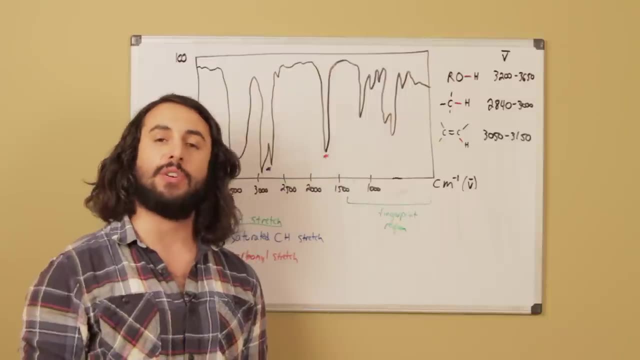 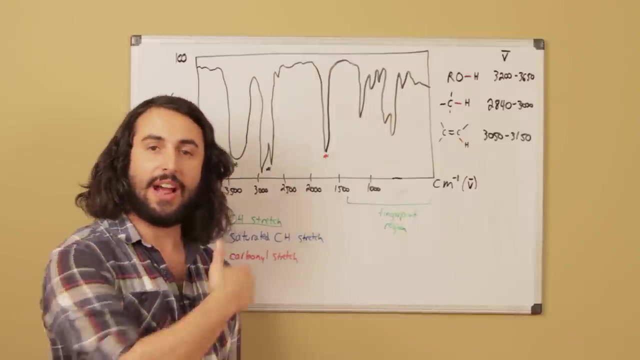 so what this means in terms of data that we can interpret from an IR spectrum. if there is an OH stretch, there is an OH group in the molecule. that means there is a hydroxyl group somewhere in the molecule. we can look at the spectrum and be very confident that there is a hydroxyl group in this molecule. now 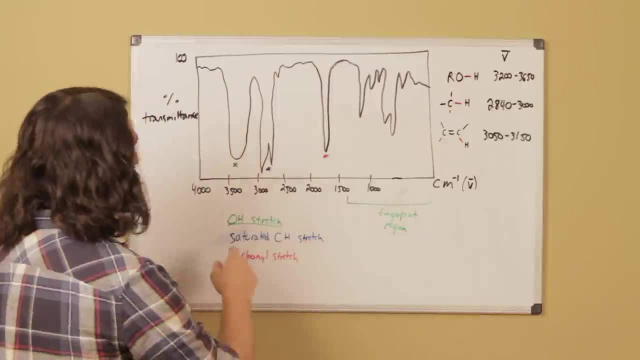 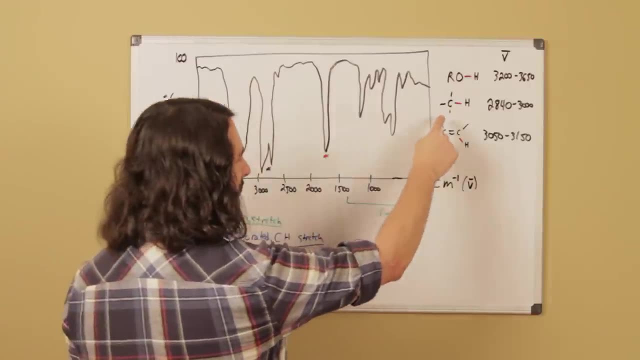 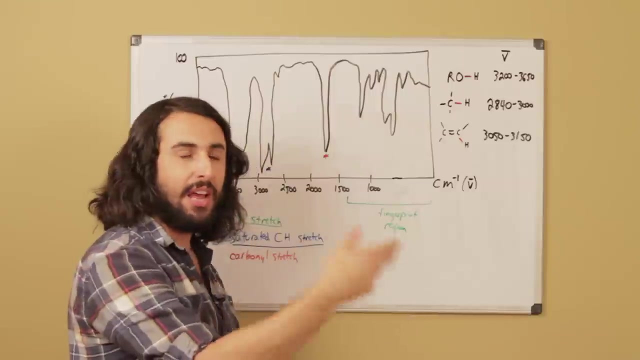 there's a couple others. we'll just look at the three most basic ones. the next one is called the saturated CH stretch. so the saturated CH stretch means that there is fully saturated carbon bound to a hydrogen, meaning this is not an sp2 carbon, it is not an sp. 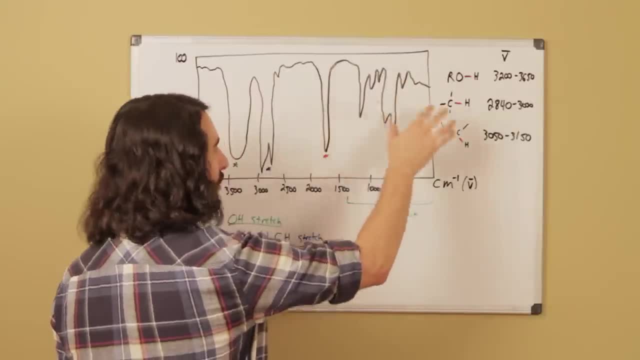 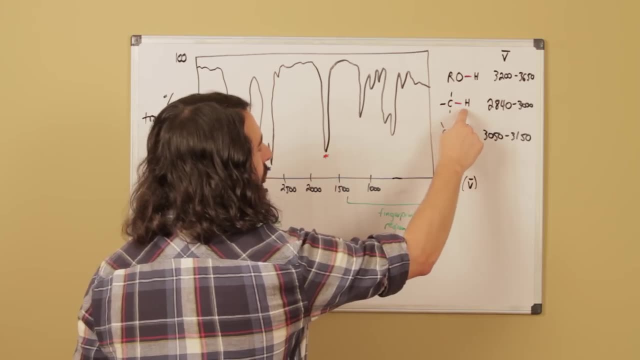 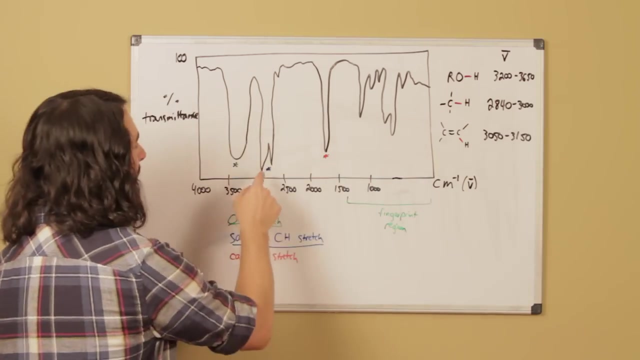 carbon. this is a fully saturated carbon, so it has maximum bonds to other carbons and hydrogens. and so this carbon-hydrogen bond, if it absorbs IR light of that wave number, it will begin to stretch, and so it's not all making it to the detector, and so 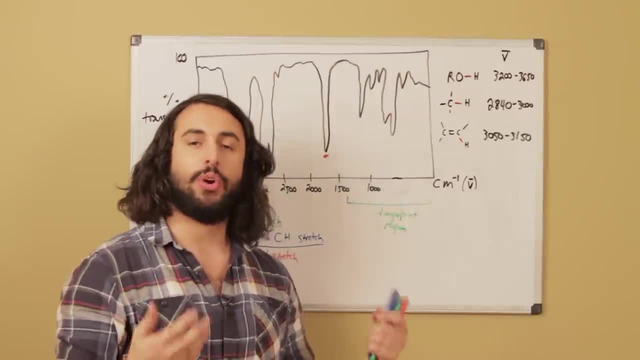 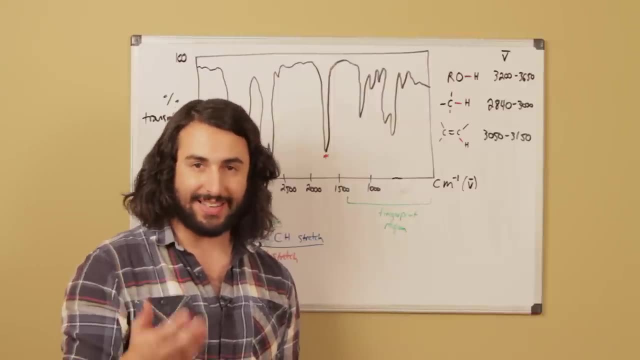 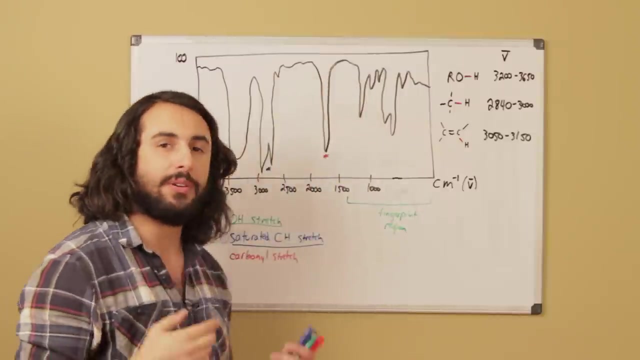 that's there, and most organic compounds will give you a saturated CH stretch, because most organic compounds have some saturated carbon-hydrogen bond in it. ok, and then, lastly, let's look at the carbonyl stretch. now, this may vary depending on whether it is a carbonyl from an aldehyde, ketone, ester amide or 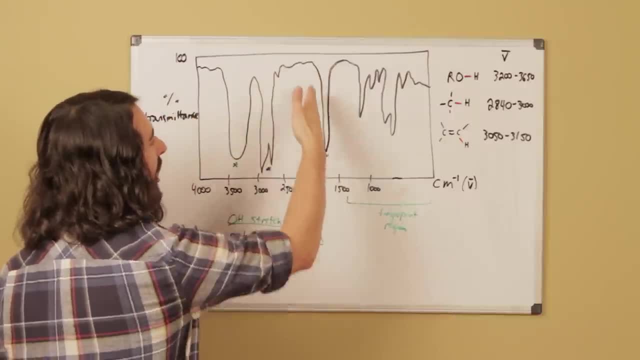 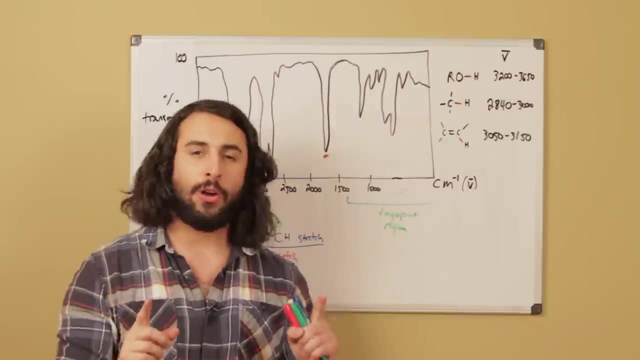 what have you, but it will generally occur somewhere in this region and it will look somewhat like this, and so if we have that stretch, we know that there is a carbonyl. now, the last thing that we want to point out, a very common error is: 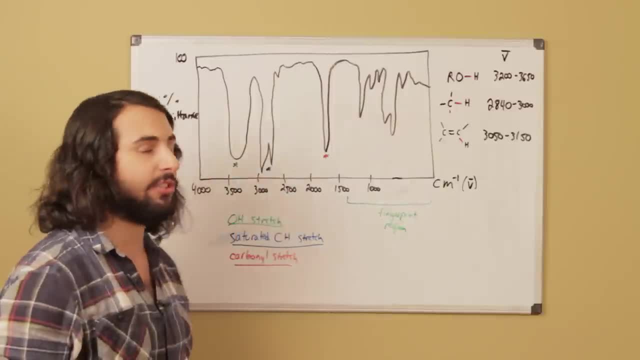 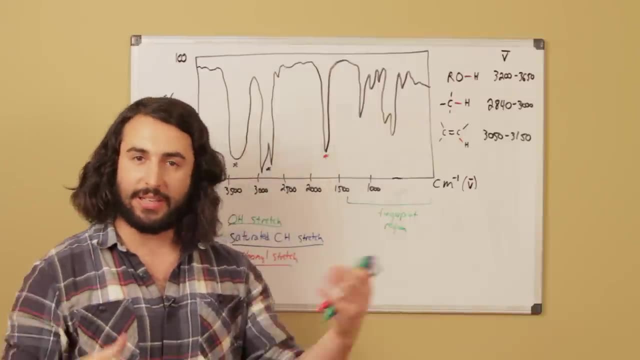 that people will say: well, there's a saturated CH stretch, so that that's the only functional group present in the molecule. or they will say there's a OH stretch, so there can't be some other functional group. all we are trying to understand is that every functional group in the molecule 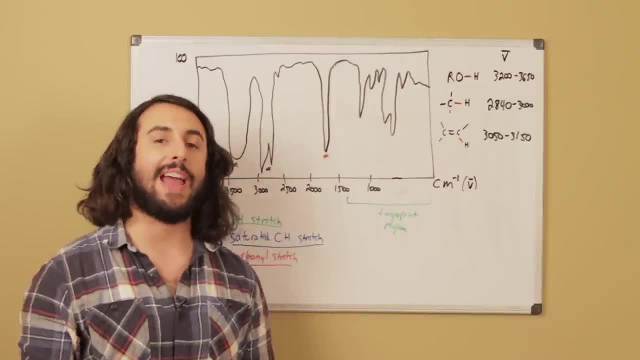 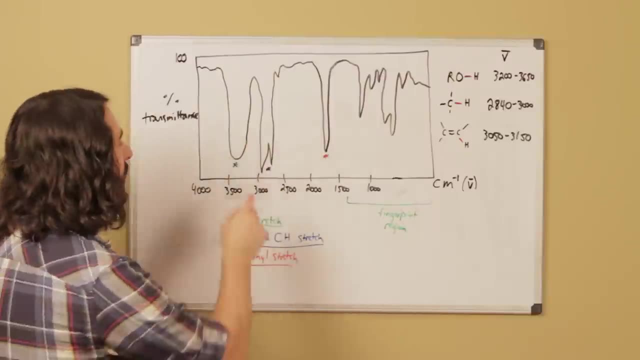 will be represented on the IR spectrum. so let's just say, hypothetically we had a molecule that gave us the spectrum, we would know that there is saturated carbon-hydrogen bonds, we know that there's a hydroxyl group and we know that there's a carbonyl of some kind. so that could look like anything. it doesn't. 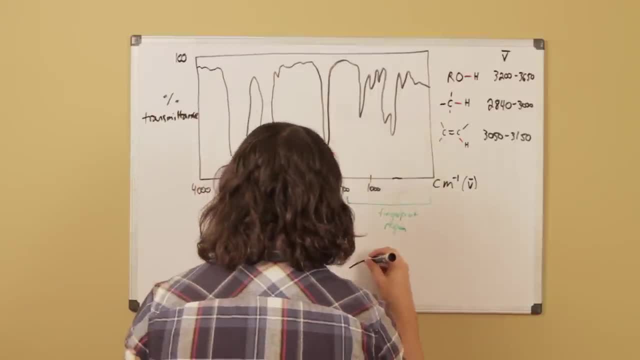 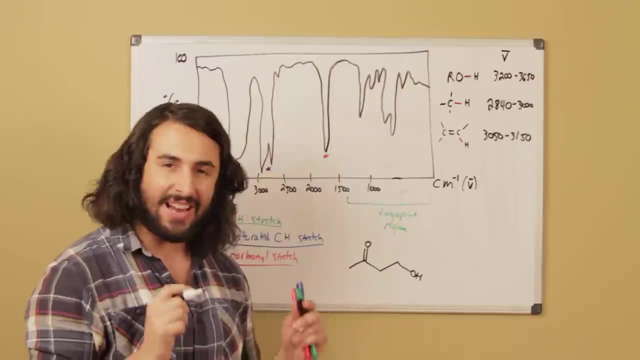 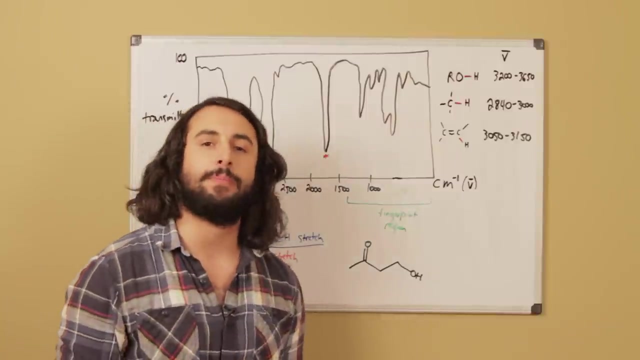 tell us the precise structure of the molecule, but it could look, say, like this: it could have a hydroxyl there and it could have a carbonyl there. we're not sure. right, it's not telling us the precise structure, but the reason this could be useful is that, let's say, we do some reaction in 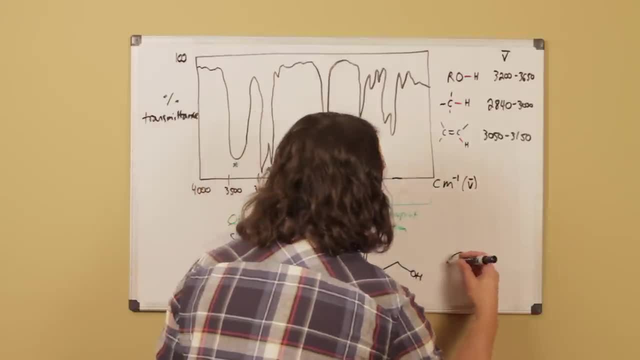 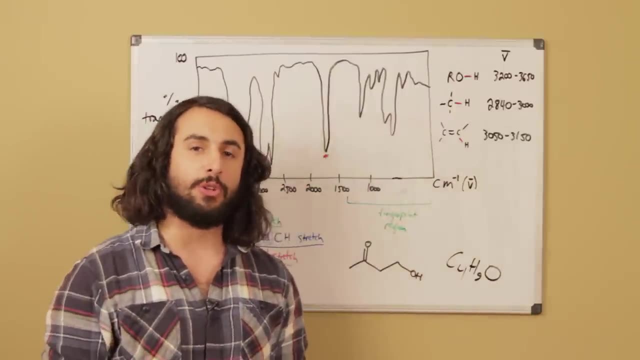 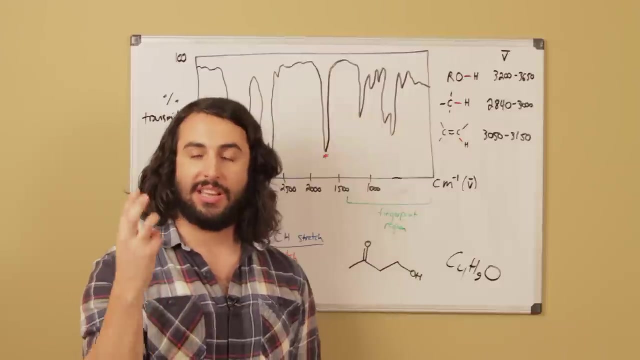 maybe we even know the empirical formula of our product and we know that our compound has an oxygen atom in it. well, the reason IR would be useful for that is we would say what kind of oxygen is it. is it a hydroxyl oxygen? is it an ether oxygen? is it a carbonyl? 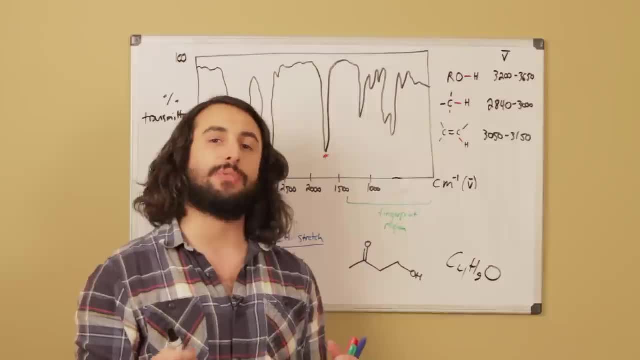 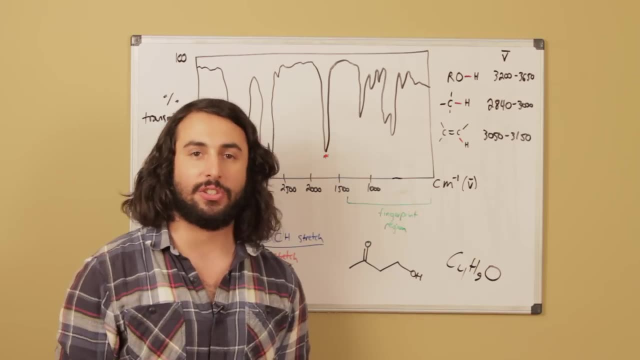 oxygen and we might get an IR spectrum and know just from that at least what kind of functional group the oxygen is participating in. if we saw an OH stretch, we would say that oxygen must be a hydroxyl oxygen. if that was not present, we would know that it is not. 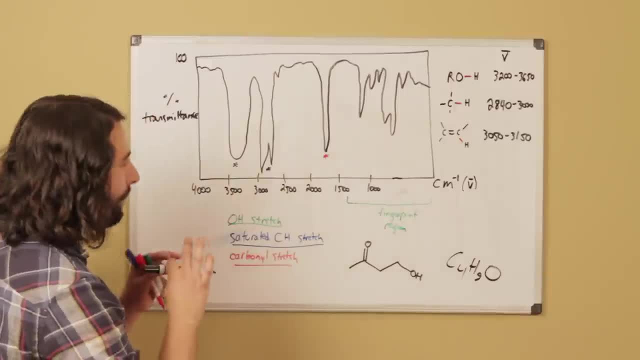 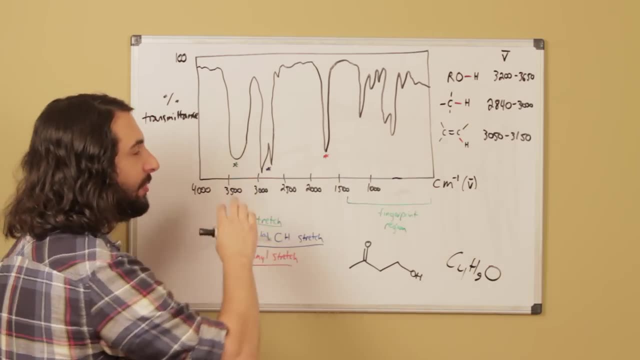 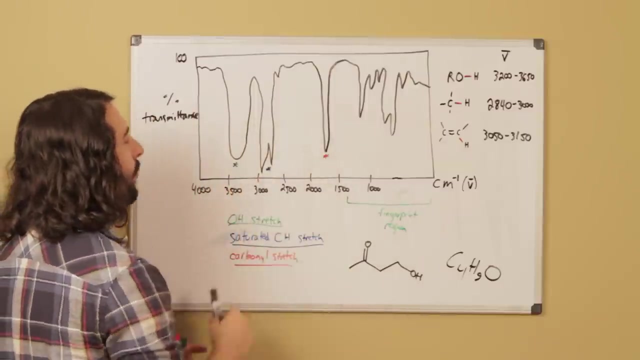 that it is not a hydroxyl oxygen. so the main thing that we want to get from this very basic introduction to IR spectroscopy is that functional groups that absorb IR light at specific wave numbers will provide very specific peaks. not only are they occurring at specific wave numbers, but they have 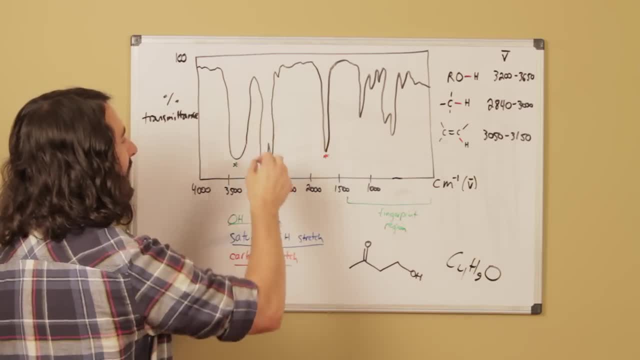 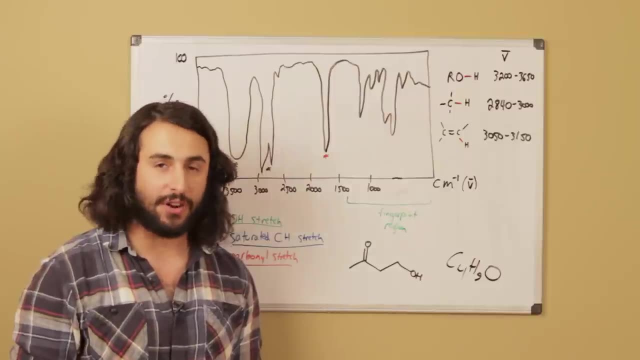 characteristic shapes. the OH has a nice curvy dip like this. the carbonyl is thin and long, and so we can take an IR spectrum and we can know roughly what kind of functional groups are in a molecule. thanks for watching. guys. subscribe to my channel for more tutorials and as